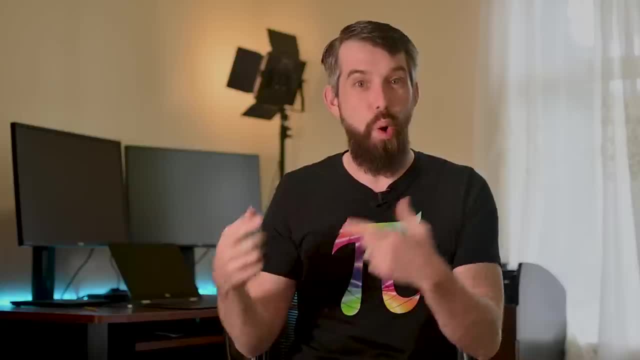 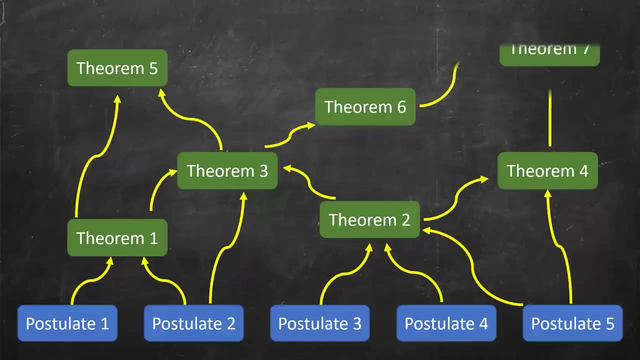 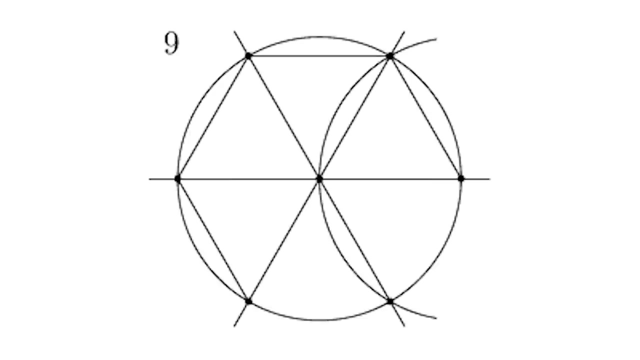 there are five of them, then everything else that you do, all of those are going to be theorems, where you try to prove theorem after theorem based on the five underlying axioms that you've accepted, For example that hexagon construction we saw earlier. This is just theorem number 15 of book four of Euclid's book, but 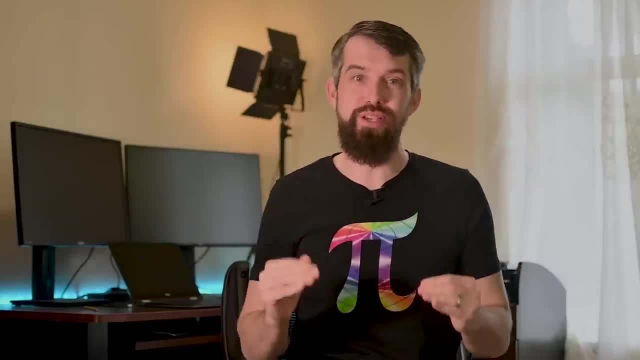 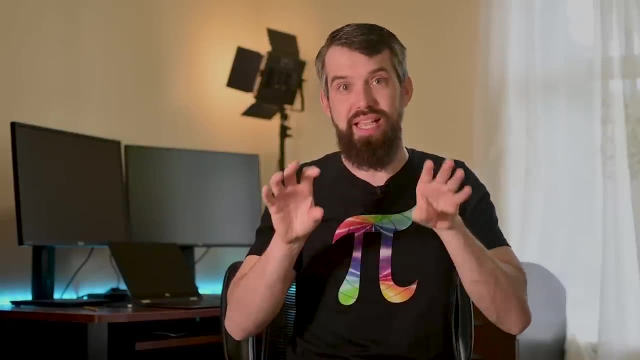 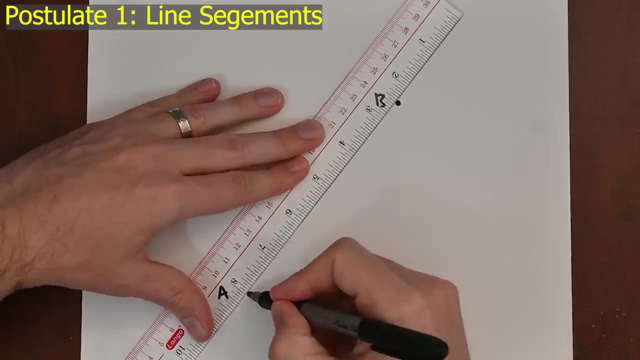 elements all proven based on those underlined postulates, And so you get this kind of enormous mathematical edifice from these underlined, very obvious and basic assumptions that we just make the choice to accept. Okay, so we saw the first postulate already, that between two points you can draw a line segment. What? 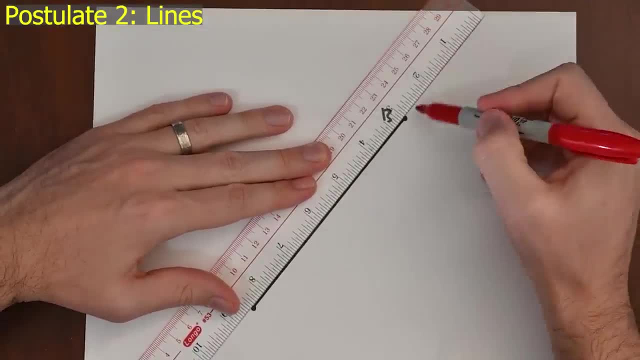 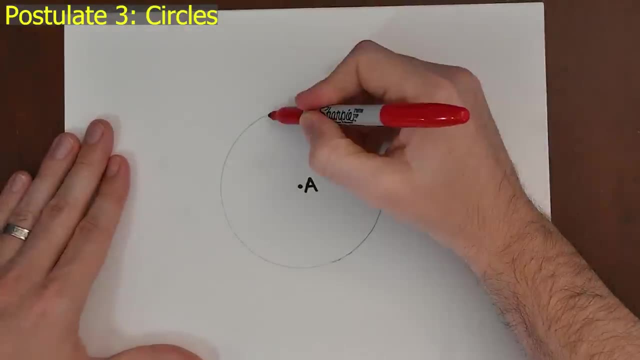 are the others. The second is that if you have a line segment already, you can extend it as far as you wished into a line. The third says that, given a central point in some radius, you can draw a circle. The fourth is that right angles, 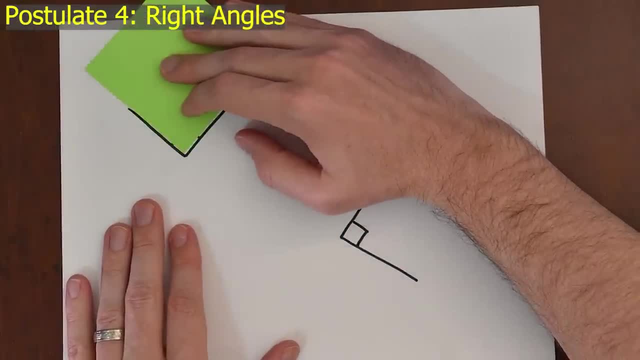 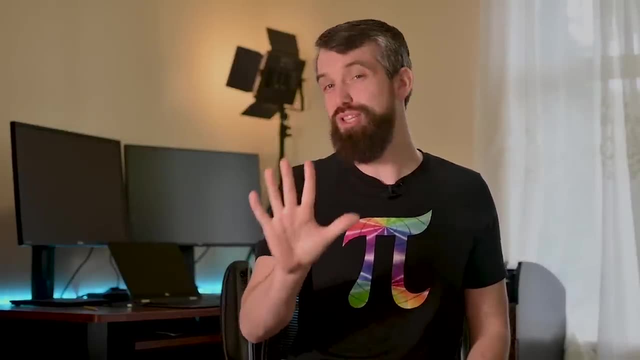 are right angles, but no matter where you draw them, all right angles are the same. So all four of those axioms are just pretty straightforward, very reasonable things to accept. But the fifth postulate, that's where it gets a little bit weirder. The fifth postulate says the following: If you start with a line and 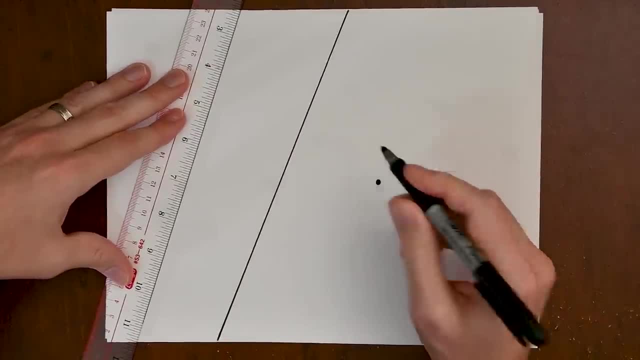 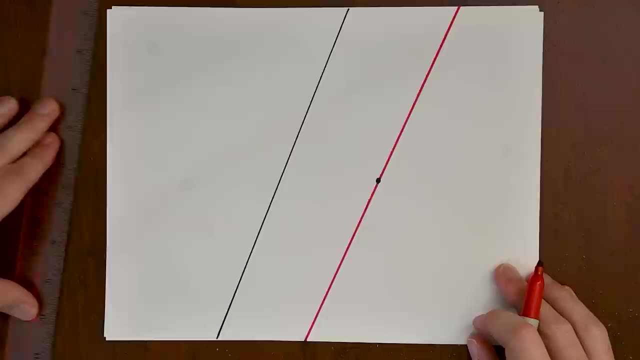 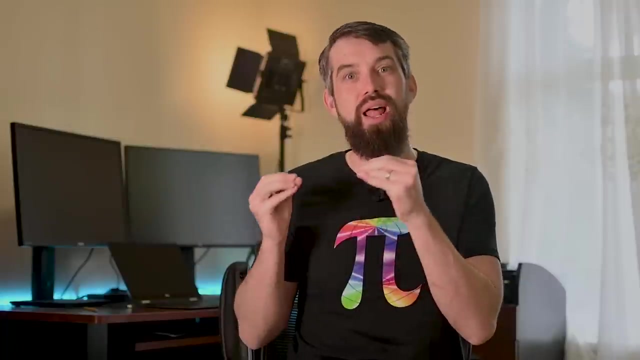 then you consider some point that is not on the line, then there is at most one other line that is going to never intersect the original line. That is, we're saying: given some starting line, you could always construct a parallel line to it And it's. 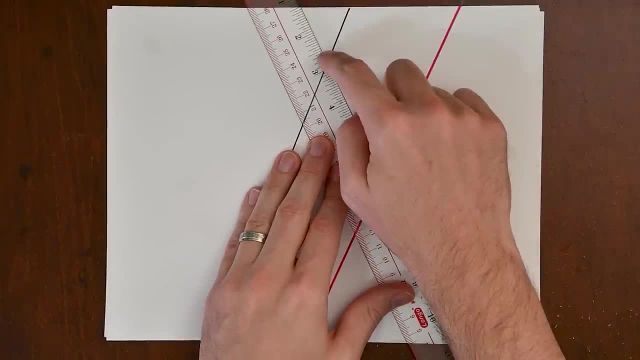 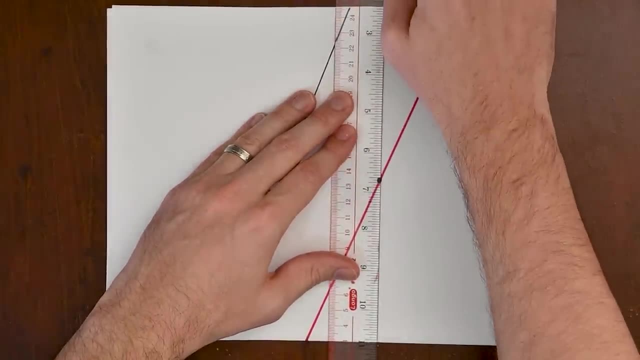 reasonable right? If I tilt my ruler a little bit, I see that the other lines that I might draw are either going to intersect the original on the page or you can sort of imagine that they're going to intersect the original, you know. 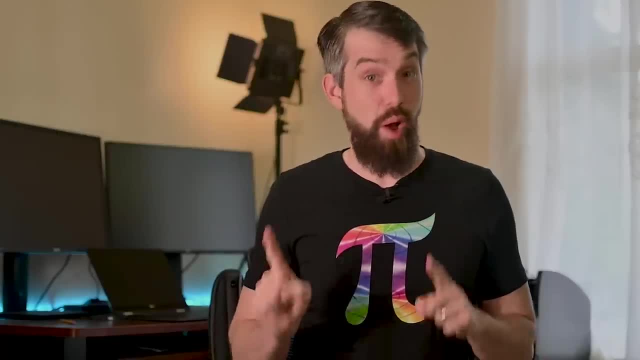 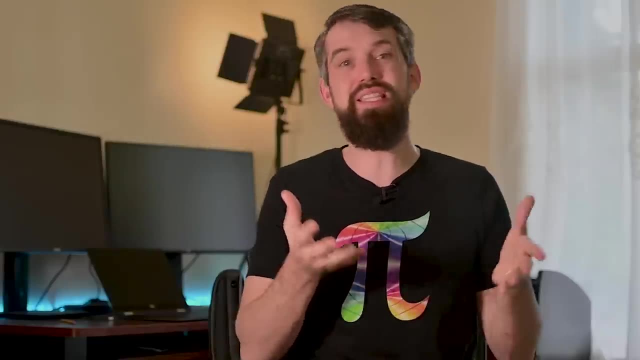 somewhere off of the page. So this fifth postulate, which we often call the parallel postulate- it's not that it's completely unreasonable, I mean it's still sort of intuitively seems like that's probably true, but it's more cumbersome, more. 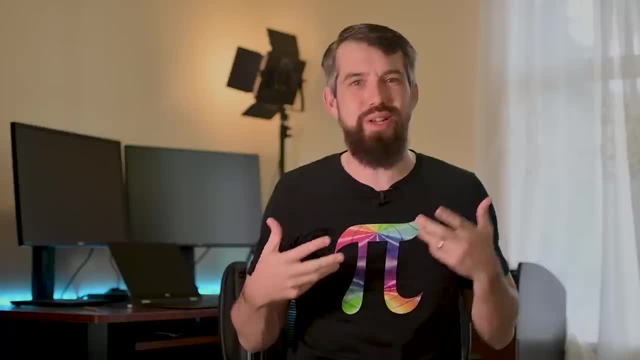 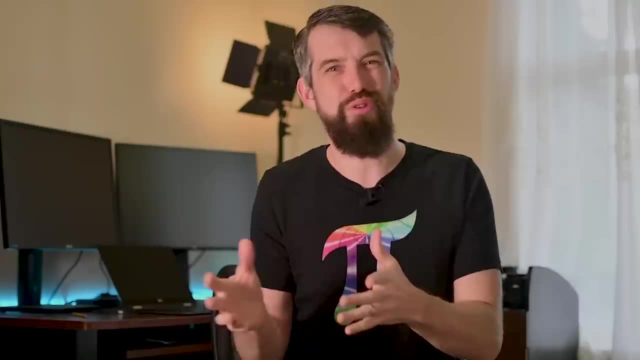 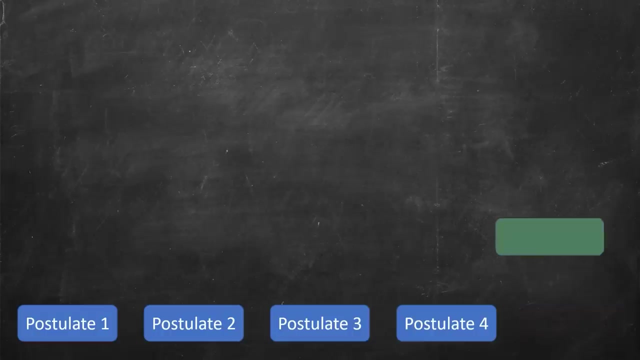 involved than the other postulates. It's some claim about what's going to eventually happen at some point. This fifth postulate, it feels like, can't I prove that. Is that really the kind of underlying bedrock assumption I need to make, Or instead, could this fifth postulate really be proven as a theory? 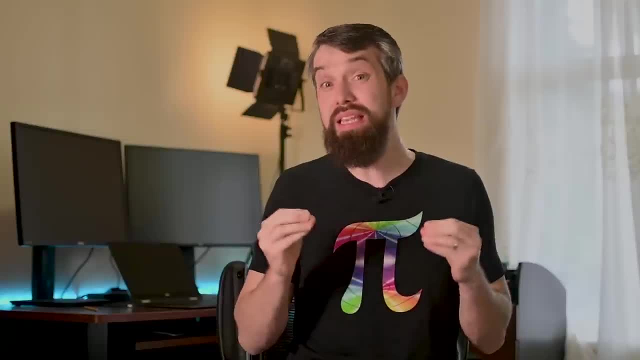 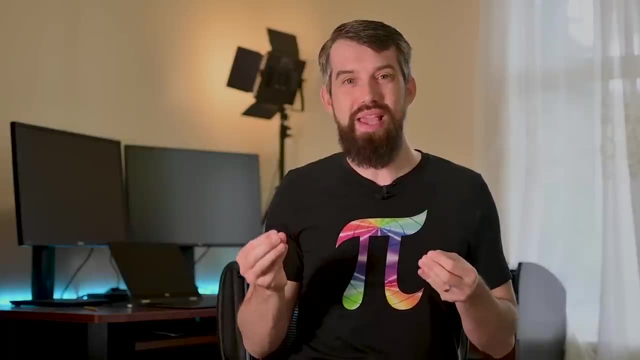 that it's simply an illusion of some sort, Or is it a theorem that depends on the previous four? Do I really need to have it here as a postulate? Even Euclid, the first 28 theorems of the elements, are all based on only those first four. 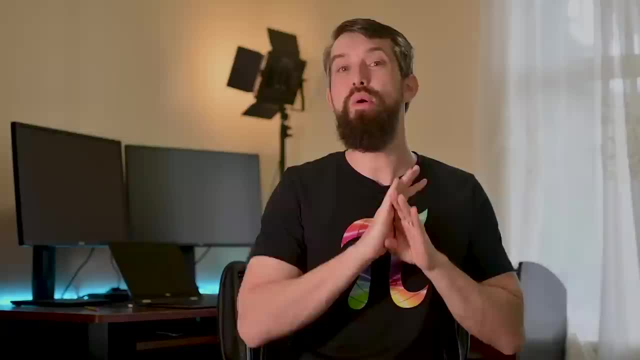 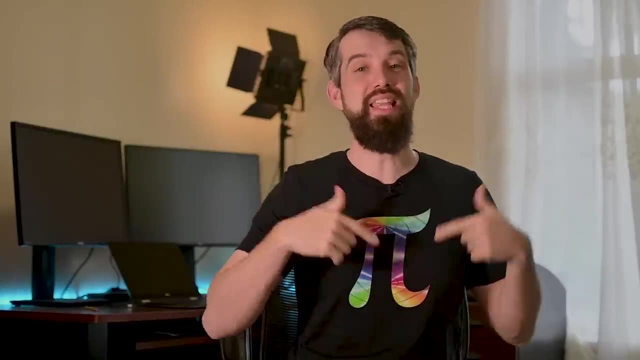 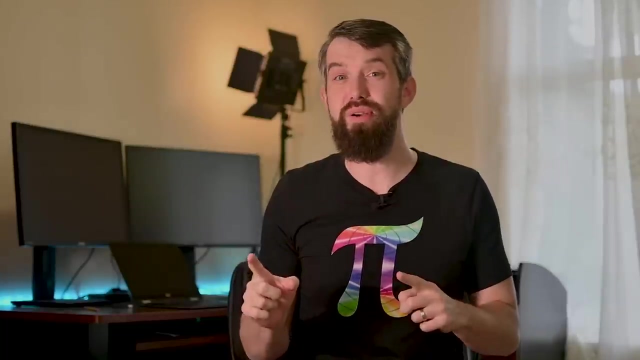 postulates. He's trying to be able to prove as much as he can without needing that fifth postulate. Now for millennia- literally millennia- mathematicians tried to prove the fifth postulate as a theorem that they never managed to do. Now to be clear, there are other geometries that 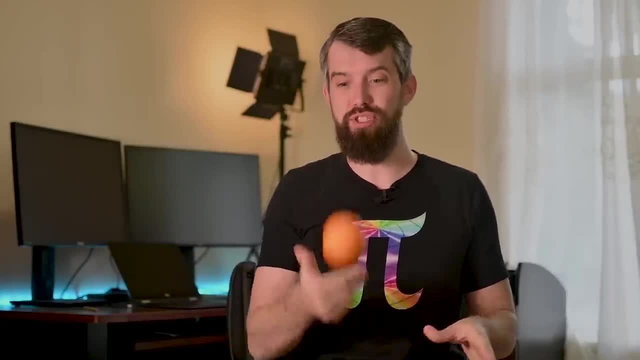 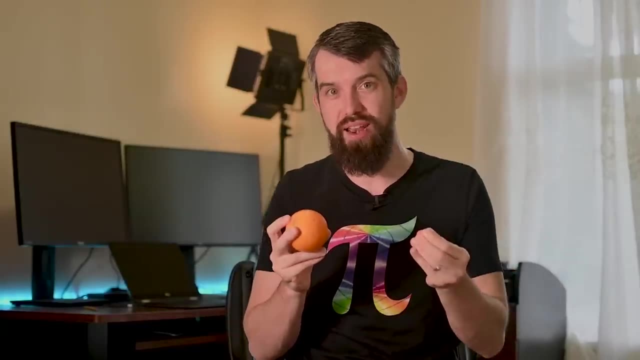 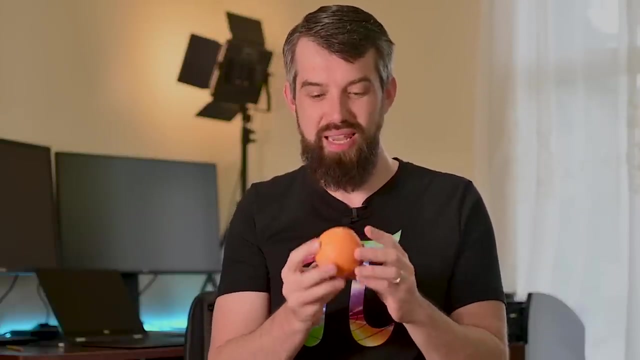 people knew about and were interested in, For example, spherical geometry, the geometry of living on the surface of a sphere, something us humans should all be interested in. If you have two points, like, say, the North Pole and the South Pole, well, what is a line between them? I'll model it with my elastic A line. 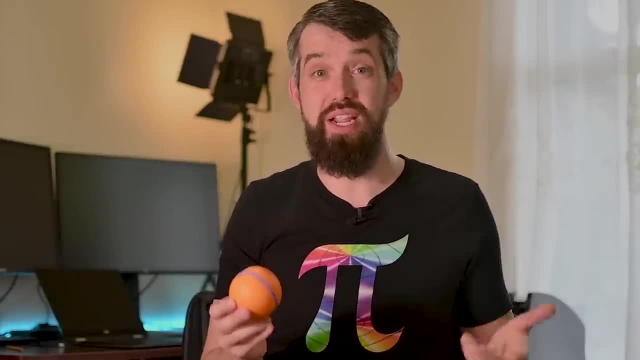 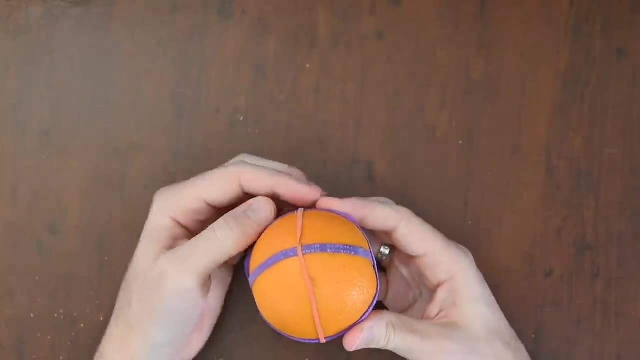 could just be a great circle or a portion of a great circle. I could add some more lines. Let's put on, for example, another great circle here, and I'll do one more again, And we can study the geometry of what it's like to live. 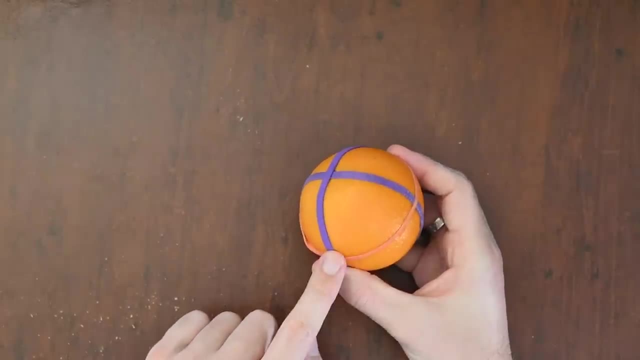 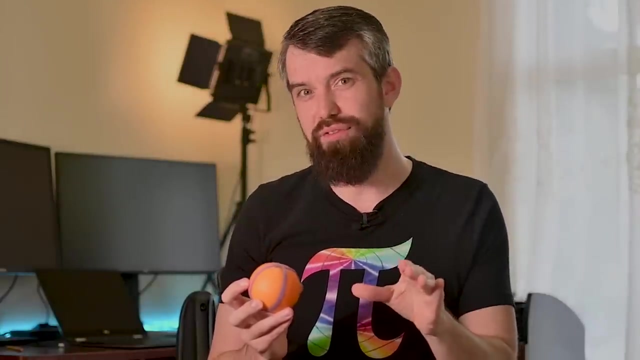 on this surface. You know right, for example, right here there's a nice little triangle and we can study properties of triangles that occur on spheres. But this spherical geometry is really different from the Euclidean geometry that we were just talking about, Because, for example, not even the first 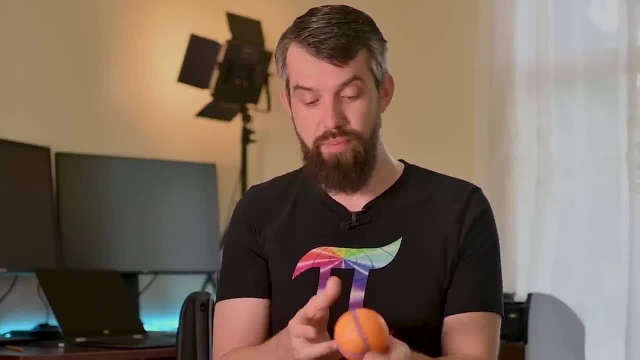 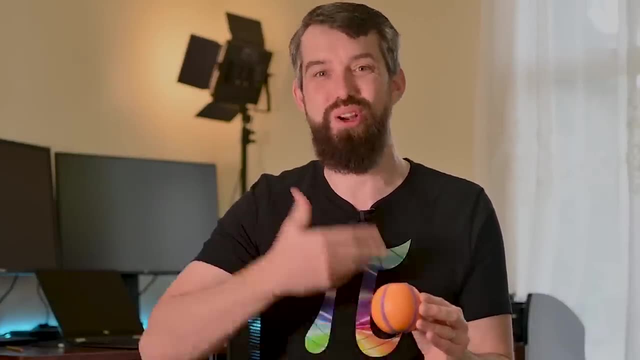 of the axioms is satisfied. If I take the top and the bottom here, these two poles, I'm going to get a little bit of a difference. We'll see that in fact there's infinitely many different ways that I could draw a great circle that goes from the North Pole to the South Pole. So 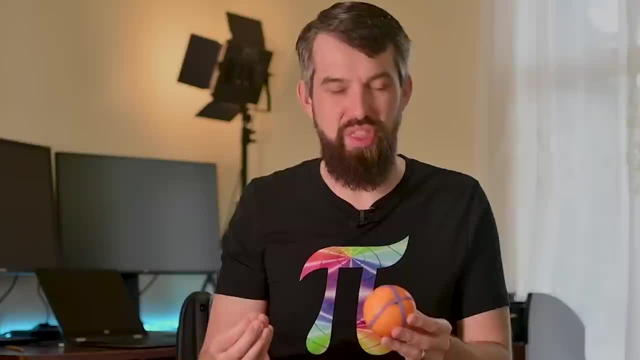 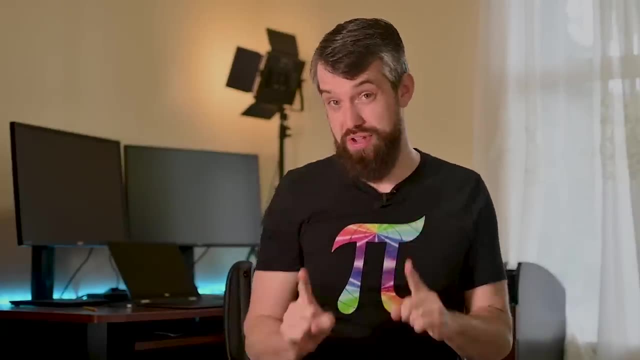 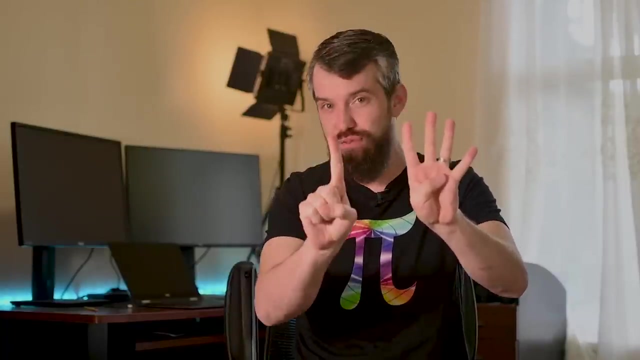 there's no way that I can uniquely define the appropriate line segment between two points. This doesn't even satisfy the first axiom. So what I really want to find is some geometry that accepts the first four axioms but rejects the fifth one, Because if I can do that, then I know that the fifth one 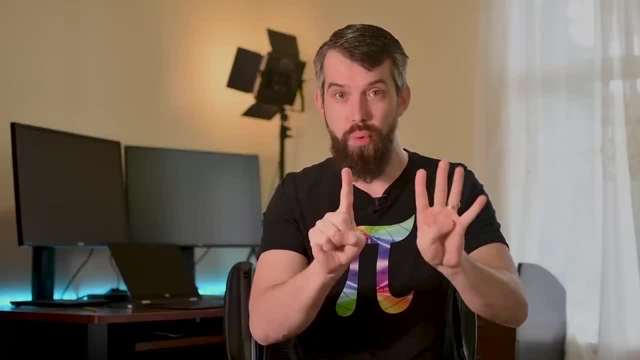 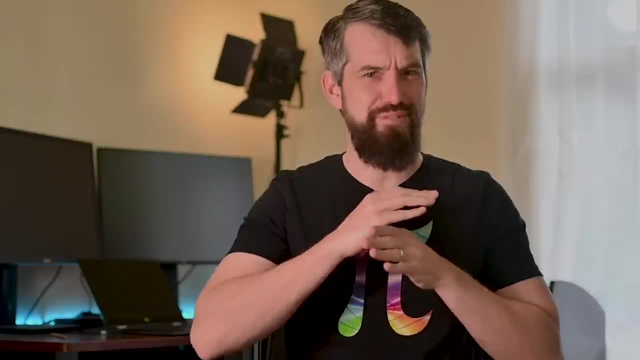 is not provable based on just the first four alone. This brings us to Janos Bolyai, a 19th century Hungarian mathematician, And Bolyai is a fascinating character in the history of mathematics, but I actually really like his father, who did. 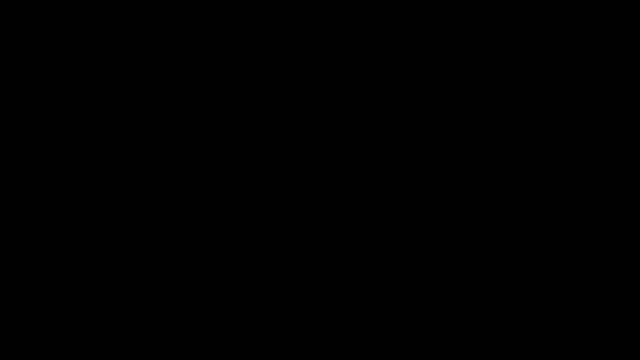 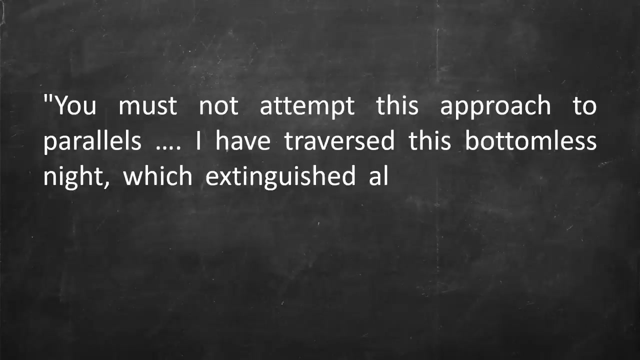 similar work before him and had this delightful quote to give to his son. You must not attempt this approach of parallels. I have traversed this bottomless night which extinguished all light and joy in my life I. I have traversed this bottomless night which extinguished all light and joy in my life. I. 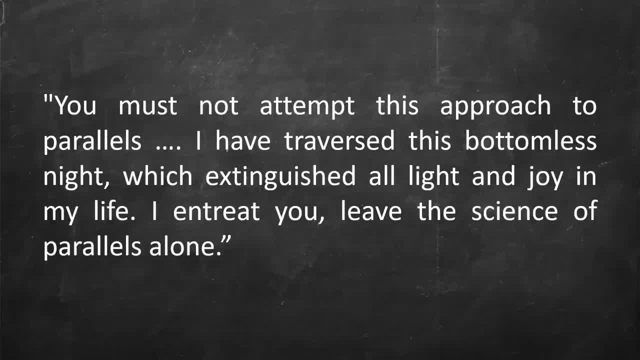 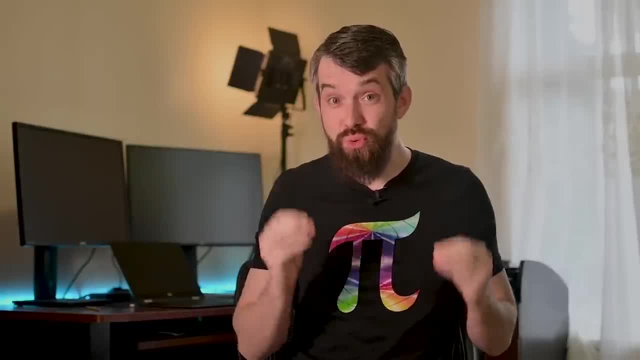 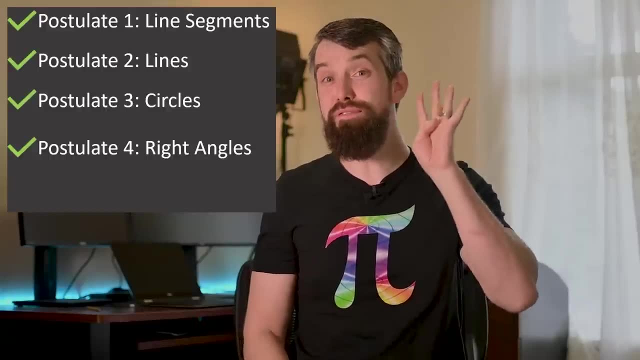 entreat, you leave the science of parallels alone. Unfortunately for us, he did not listen to his father. What Bolyai did was construct such a consistent geometry, which we now call hyperbolic geometry, that accepts the first four postulates of Euclidean geometry but rejects the fifth. This is the so-called 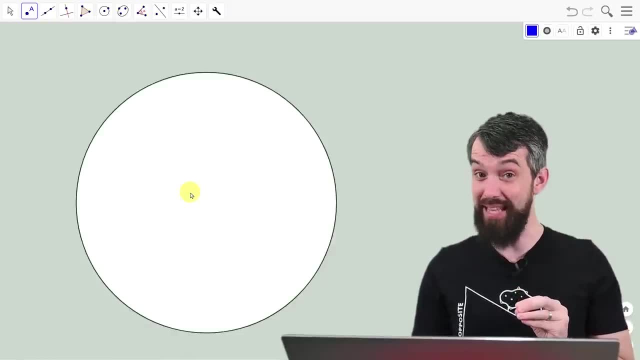 Poincaré disk, And the idea is, you can live inside of this disk, but you cannot step outside of it. You can't even step onto the boundary circle. Now what I'm going to do is I'm going to put two points, A and B, inside of my Poincaré. 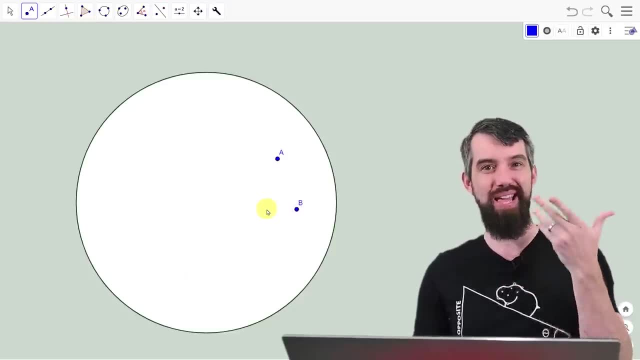 Disc And I want to try and define what do I mean by a hyperbolic line segment? I want to try and define what do I mean by a hyperbolic line segment between them, a type of line segment that was going to obey well the different. 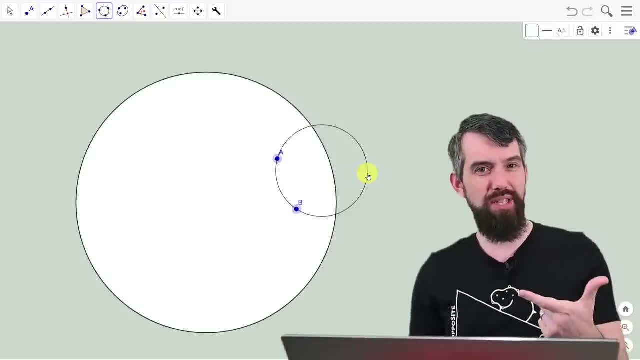 axioms of Euclidean geometry, most of them. And then one thing I know is that if I have two points, A and B, there are many different circles that lie between A and B, And all of these circles are called the Pen objectives of Poincaré. We cannot. 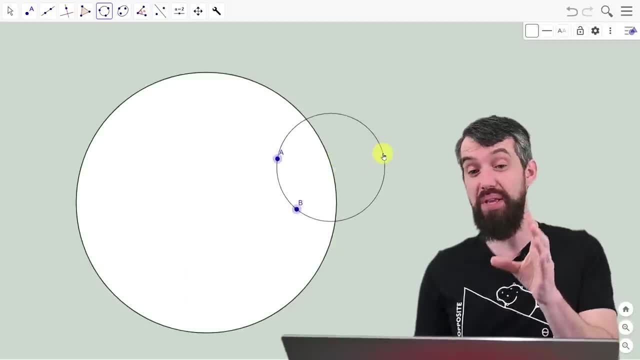 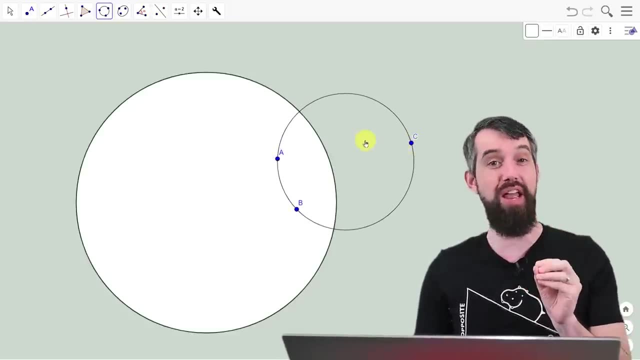 these circles are possible circles that just have A and B on them, But there is exactly one possible circle- maybe it looks somewhere around there- where the intersections there and there with the boundary circle form 90 degrees. So that is to say there are many different circles between two. 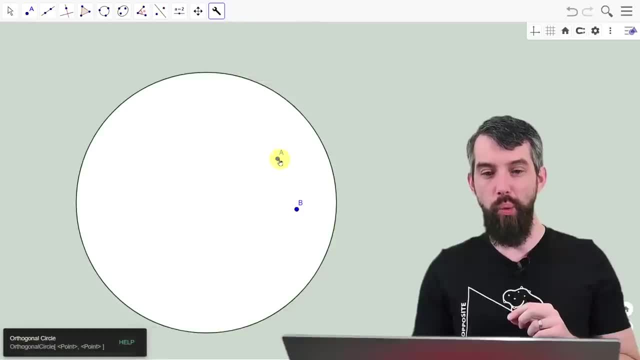 points, but there is only one orthogonal circle between these two points, Orthogonal in the sense that it comes and intersects the boundary circle at 90 degrees. Now, I'm doing all this, by the way, using software called GeoGebra- the link is down in the description- and I've taken standard GeoGebra. 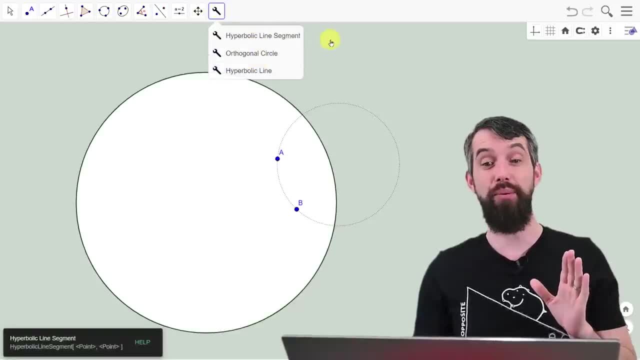 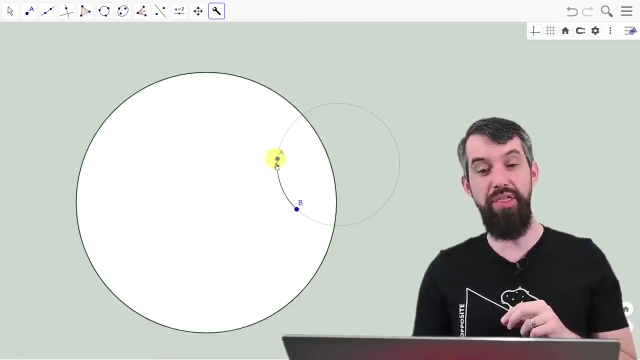 and I've customized it with a few special tools that will allow us to do hyperbolic geometry really nicely. So now I'm going to define what I mean by a hyperbolic line segment. So I click the hyperbolic line segment button and I'm going to select A and B here and basically this portion. 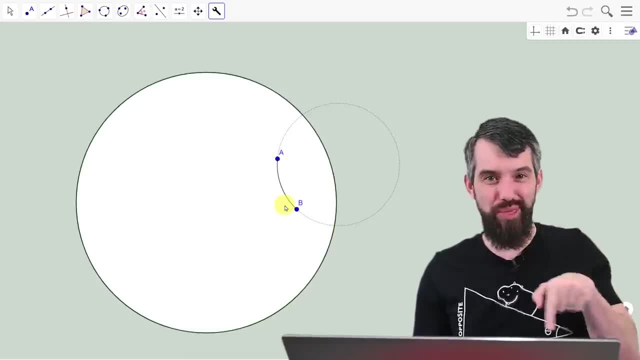 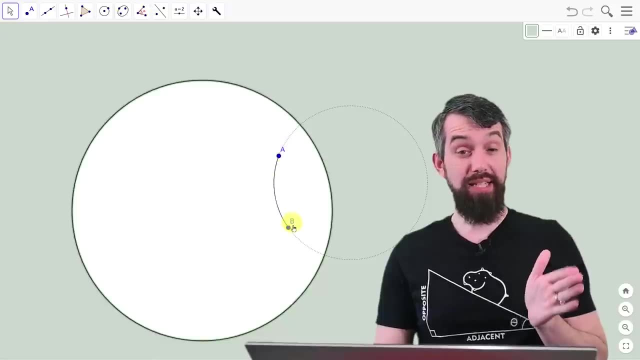 this portion of that special circle, this orthogonal circle that goes between A and B. I'm going to call that a line segment in hyperbolic geometry. This gives me the line segment. If I want to give the actual line, I'm going to go and click hyperbolic line between A and B and it extends it all the way out. 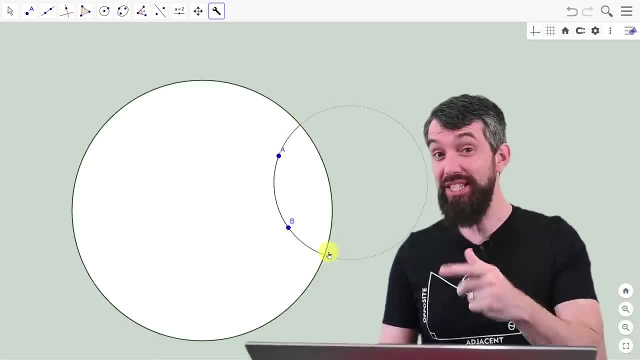 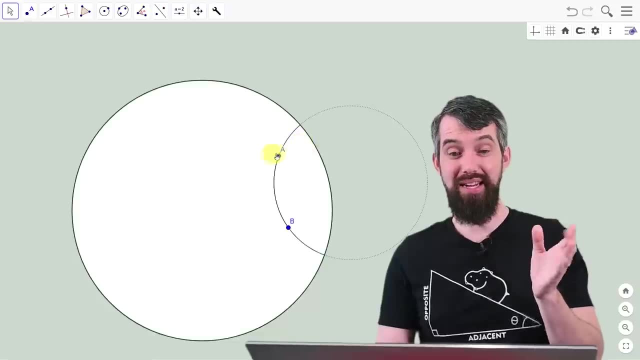 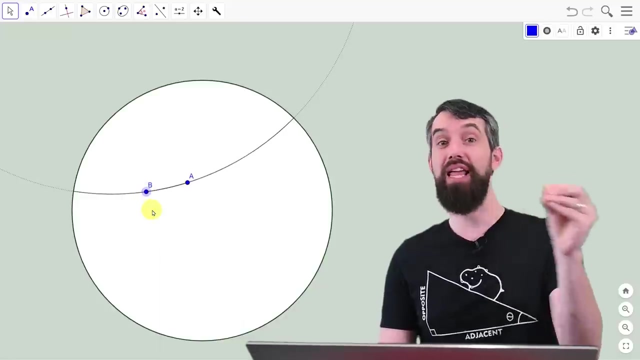 to the boundary circle. So what we've established is the first two postulates that Euclid came up. between any two points, I can come up with a line segment between them, and it doesn't matter how I move my points around, No matter what I do with the A and the B, there's always a uniquely defined line segment between them. 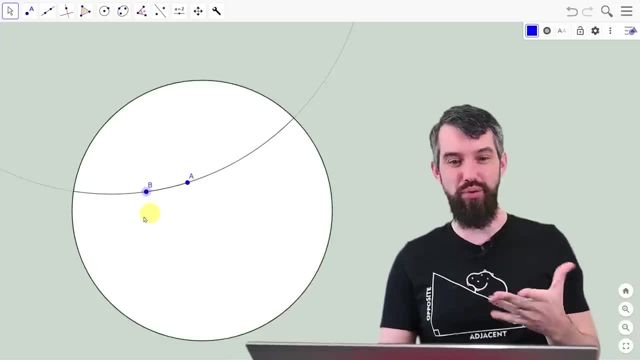 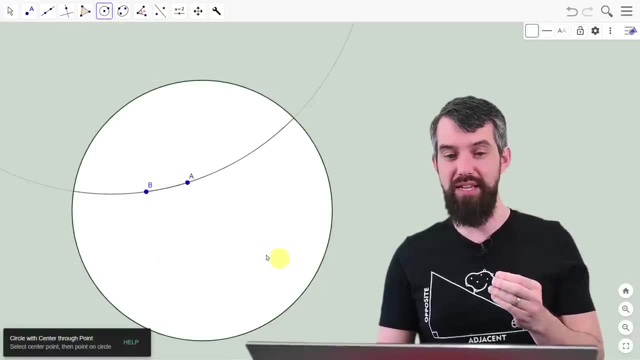 Second postulate is that, given a line segment, I can extend it into a full line. This is my definition of a full line and again, I can do that. I can also come up here and give the idea of a circle. A hyperbolic circle is just a Euclidean circle, There's no difference. 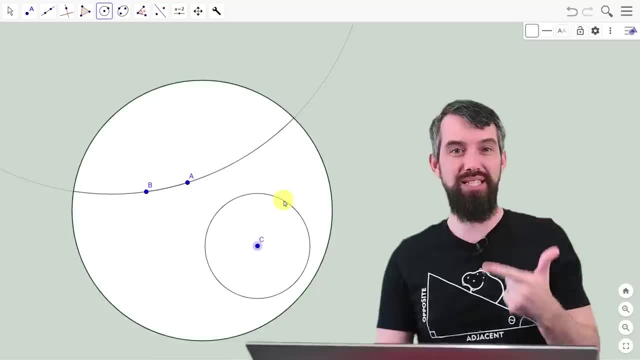 except for the restriction that the hyperbolic circle has to live fully inside of the Poincaré disk. I can't have something like this, where part of it's inside and part of it's outside. That's going to be a little bit more complicated. 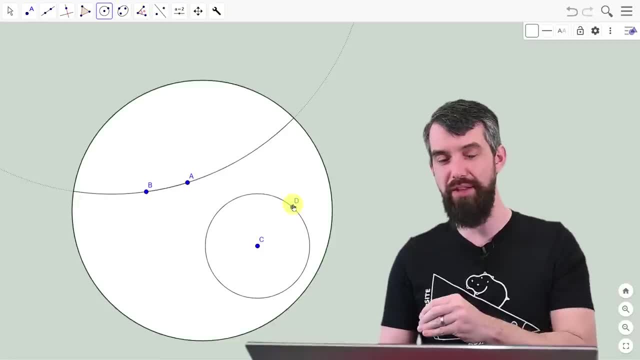 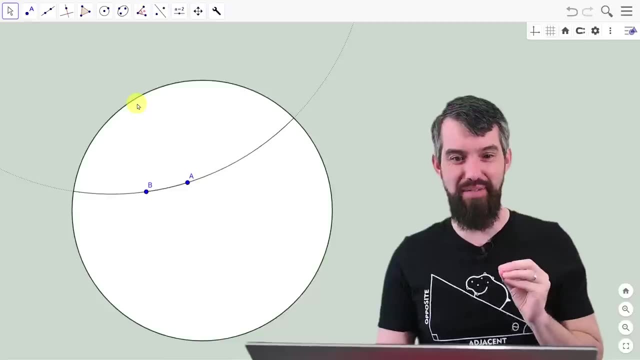 That's going to give me the third axiom. Angles, we'll talk about a little bit later in the video. But now let me talk about the parallel postulate, the fifth one. That's where all the special stuff happens, Because consider this first line that I have established already- 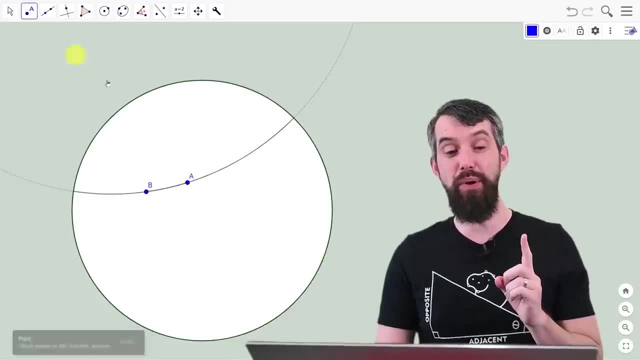 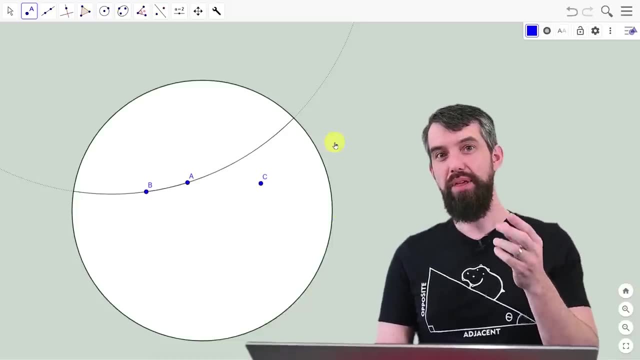 Now let me imagine that I'm going to come here and I'm going to put in just some other point. How about that point over there? I'm going to call this one C. If the parallel postulate was true, then there would be exactly one line that goes through C. 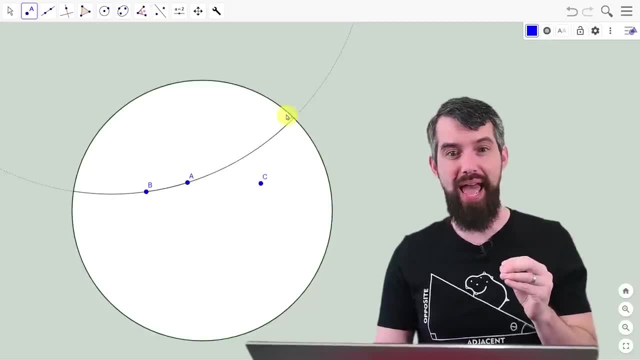 but does not intersect the original hyperbolic line that I have. But if I come here and I start at C, then what we're seeing here is that there's actually infinitely many other hyperbolic lines that go through the point C, that do not go through the original line. 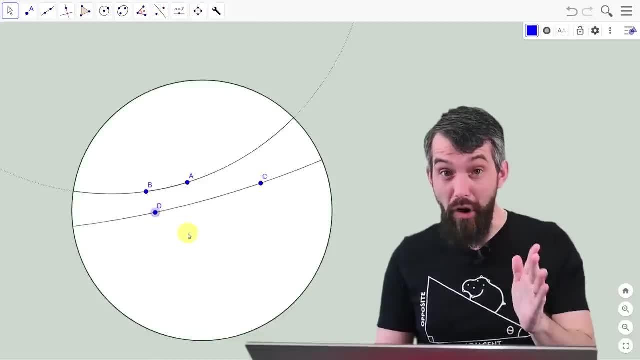 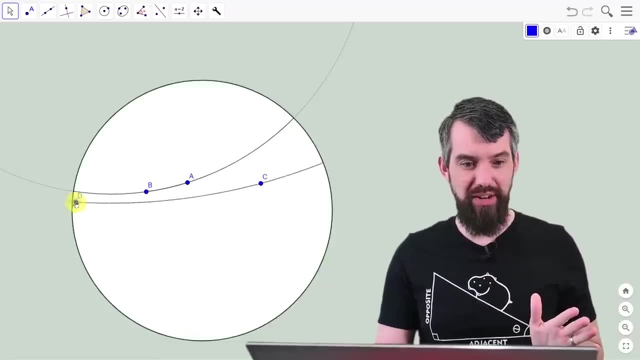 This tells us that the parallel postulate is false. There is not exactly one line that is parallel to the original. Perhaps there's a couple here that are special, For example, if I take this D point and take it right down to this intersection here. 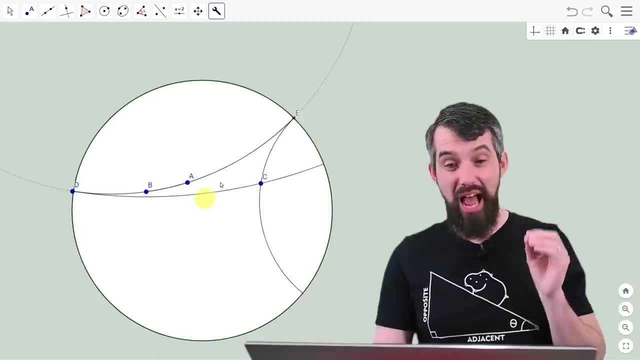 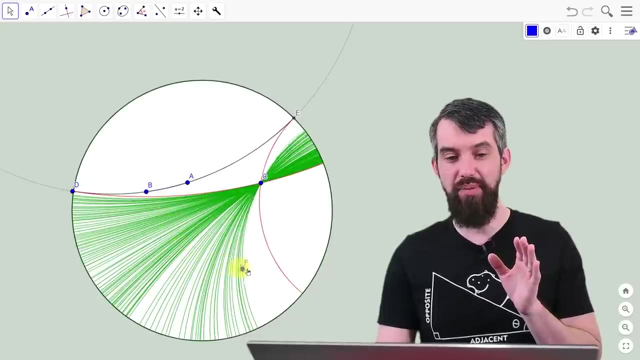 maybe this one I could call parallel. I have this other parallel line that goes between the other intersection point with the boundary circle and C. I'll make those two red just for convenience. But then if I take any curve that starts in here, any of those ones that lie in this sort of region, in between these two different red curves, 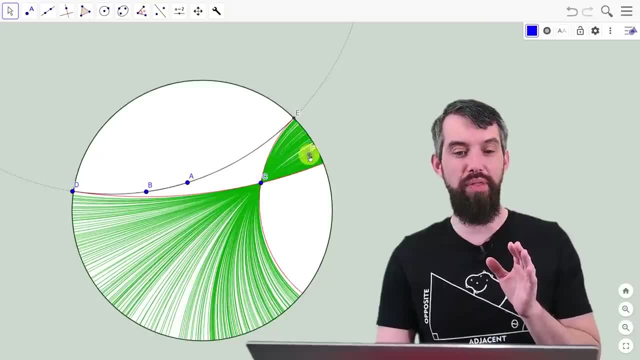 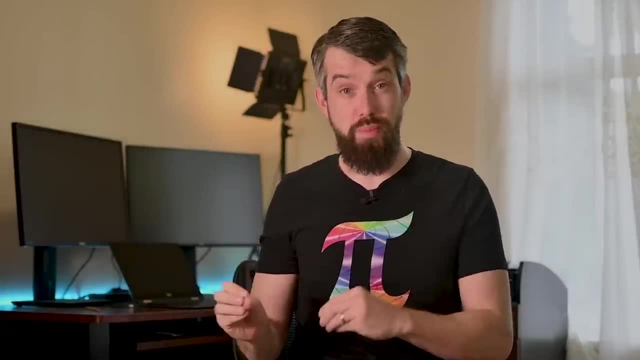 I could even go all the way up into the middle here, anywhere over there. all of those are not intersecting my original line. So what we've really done here with hyperbolic geometry is we've put that age-old question to the rest. 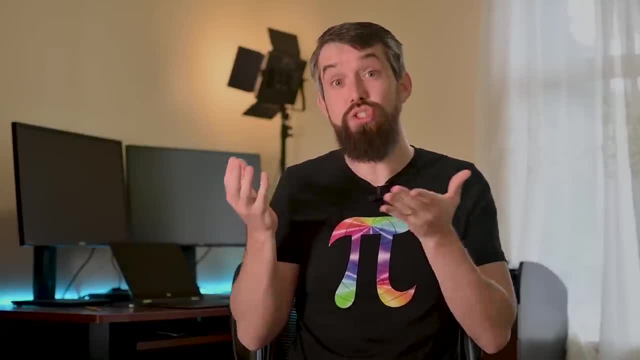 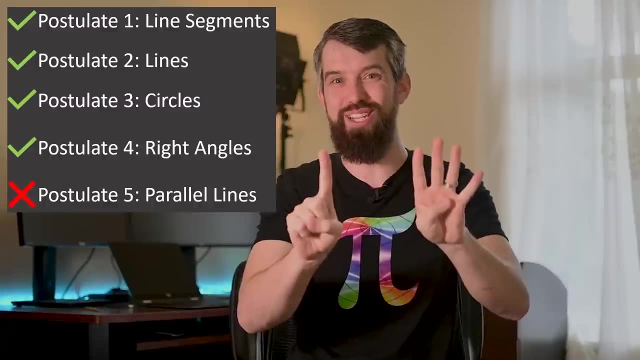 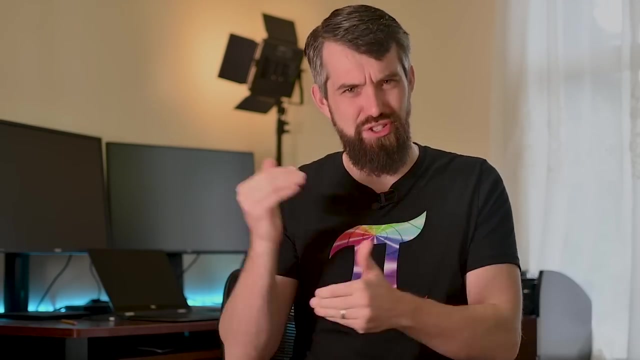 Yes, we can find a geometry, a consistent geometry, that accepts the first four postulates but rejects the fifth one, And thus that fifth postulate cannot be proven from the first four alone. To be clear, we have skipped over a lot of the hard work of showing that this geometry is consistent. 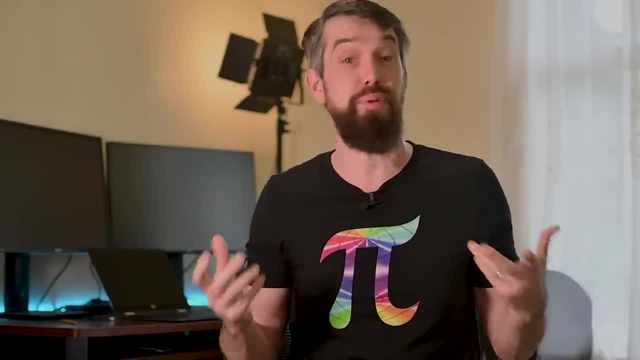 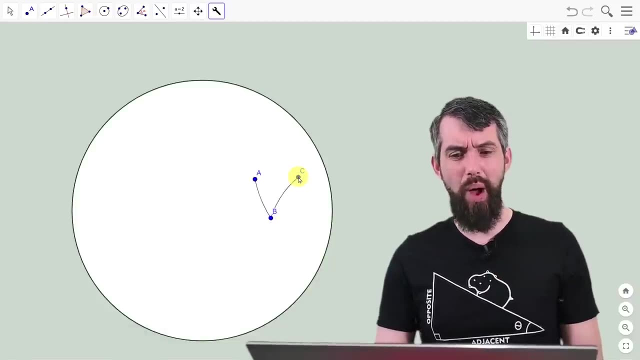 but that's what Boyaie and others that followed him were able to do. The next thing I'm going to talk about is angles. So let me imagine that I have two different lines And I'm really interested in how should I define this angle down here at this point B? 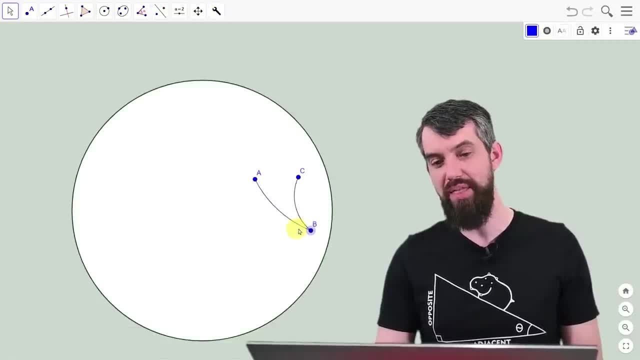 I can see, as I move it around here, that that angle is actually going to change. So the way I'm going to do this is I'm going to come up with some tangent lines. At B, I'll take a tangent line to the first curve and similarly at B to the second curve. 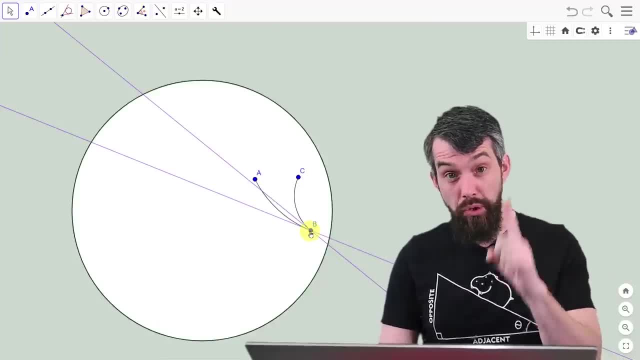 These are Euclidean lines. they're not related to hyperbolic geometry, but I'm going to use them to define something in hyperbolic geometry. So as I move my B around you can sort of see how those tangents are going to be defined. 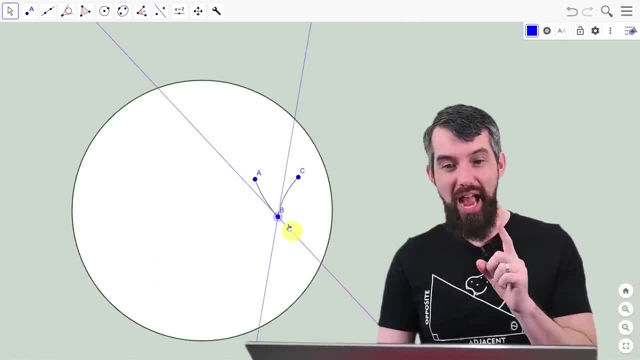 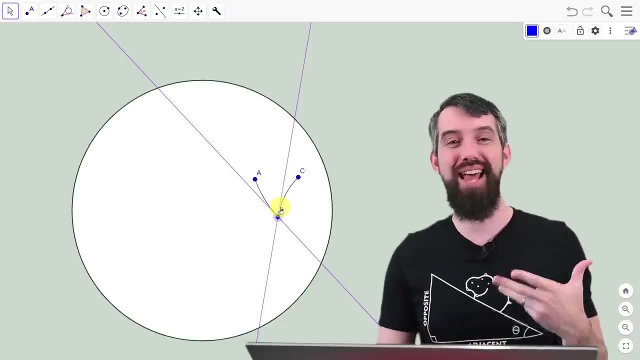 You can see how those tangents are going to be changing. Then I define the angle at B to be the angle between the tangent lines And now I have a nice definition of what the angle is, Closing this up into being a triangle. I can contrast this hyperbolic triangle. 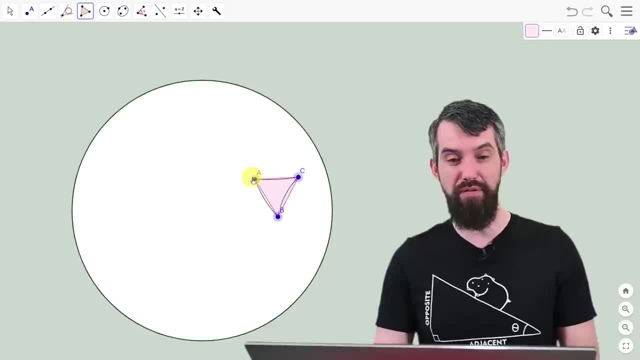 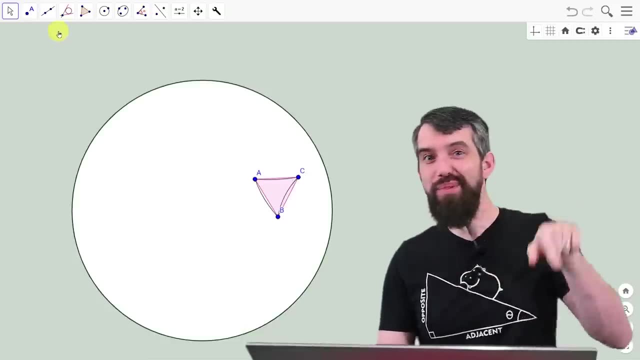 with the Euclidean triangle that could be formed by just taking straight lines, in the Euclidean sense, between these two different points. For a Euclidean triangle, we know that the sum of the interior angles always adds up to 180 degrees, But watch what happens here. 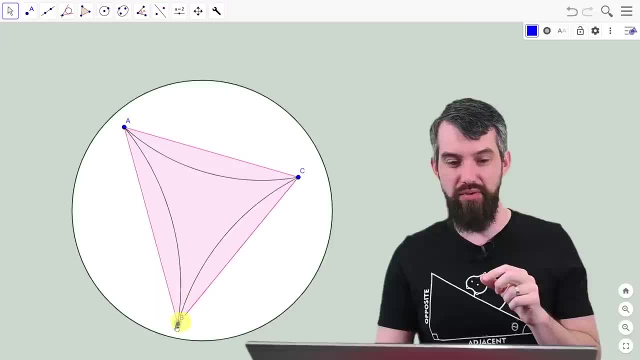 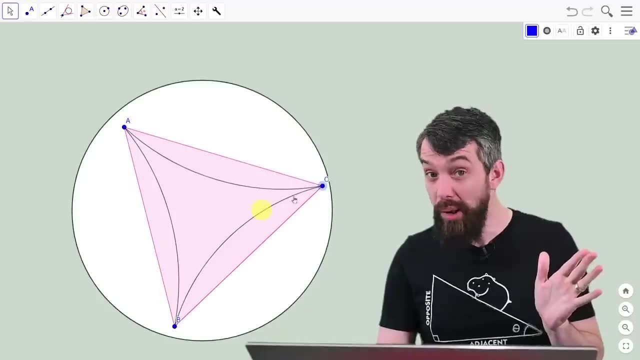 I'm going to drag the A all the way over there, I'm going to drag the B down here and I'm going to drag the C over here, just to make the difference between my Euclidean triangle and my hyperbolic triangle particularly apparent. 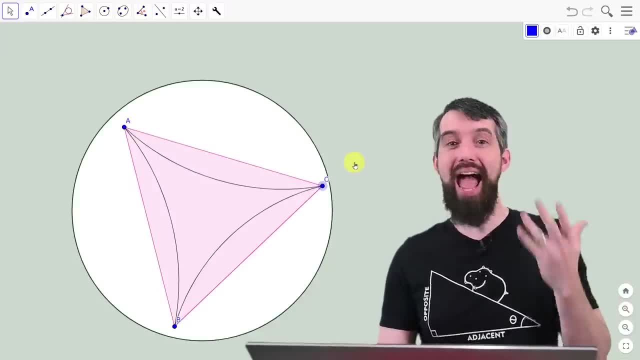 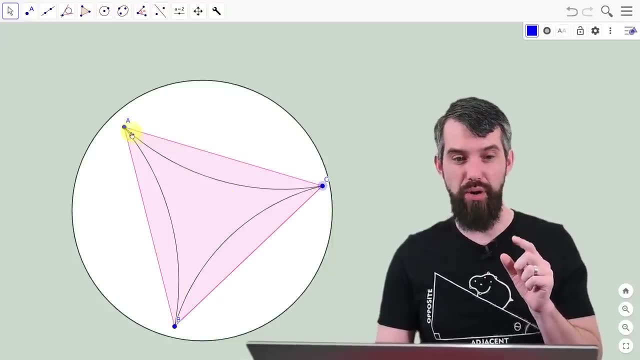 For the Euclidean triangle, the interior angles, as always, have to add up to 180 degrees. They look roughly close to 60 each in this case, But notice how small the hyperbolic angles are going to be, And indeed, if I take these all the way up, 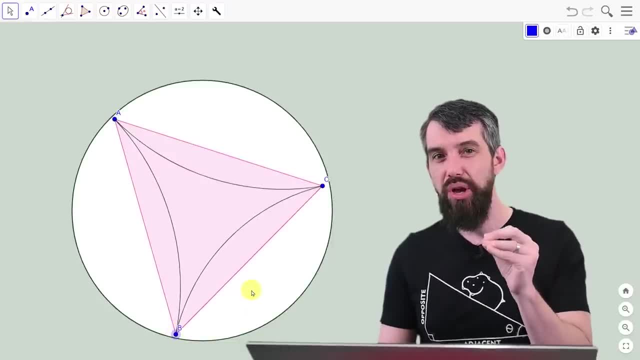 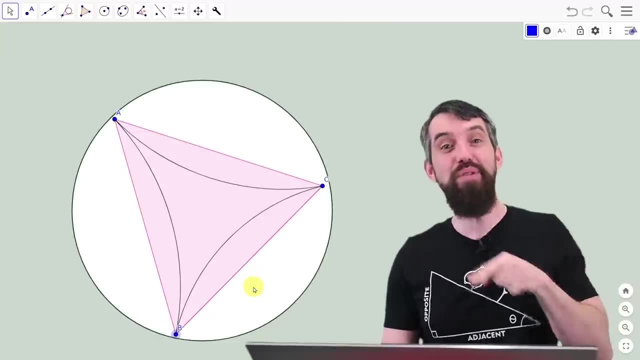 all the way to the very, very edge. those angles are approaching zero, And so, by taking the A, the B and the C and putting them as close to the boundary as I wish, I can make the sum of those interior angles approaching as close to zero as I wish. 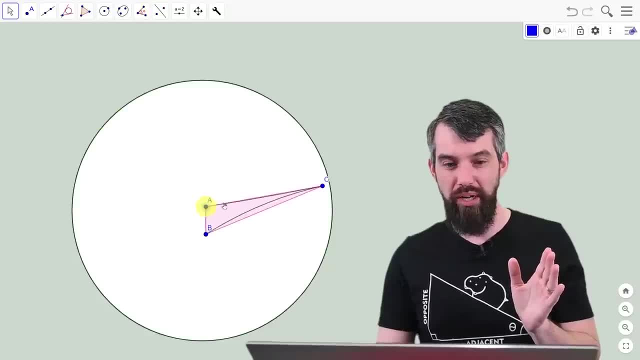 In contrast, if I come here and I put all of my points really close together and towards the center, well, I can't even tell the difference, at this level of resolution, between a hyperbolic triangle and a Euclidean one. So in this case, the sum of those interior angles. 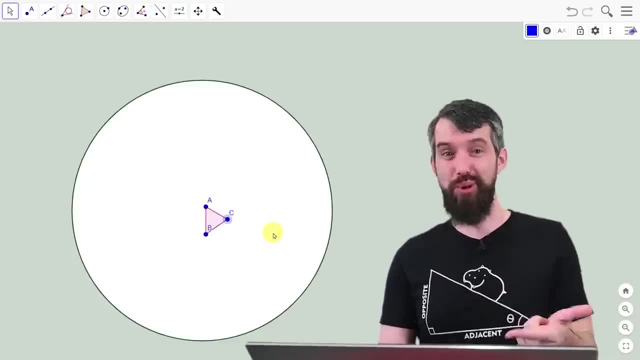 starts approximating pi. So this is just one of those quirks of hyperbolic geometry where the sum of the interior angles of triangles is not always just pi or 180 degrees. It can be all sorts of things between zero and pi at the outer edges. 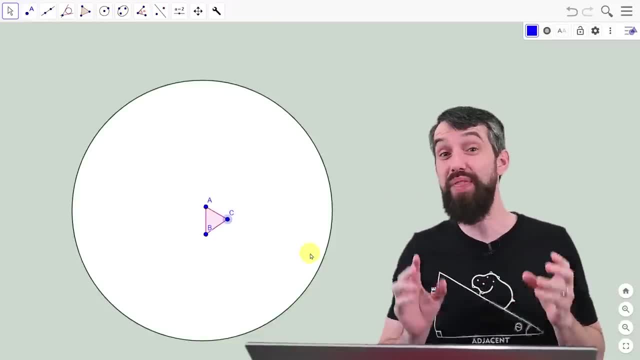 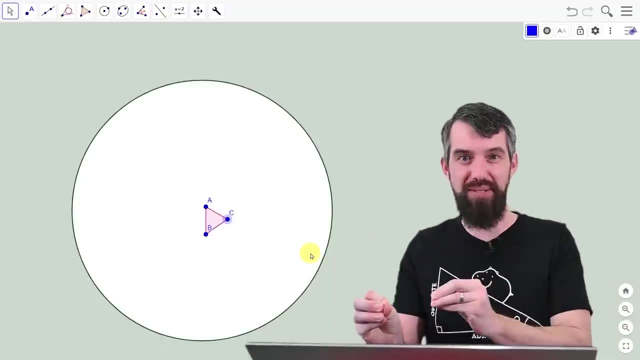 So this is just scratching the surface of what we can talk about with hyperbolic geometry, but it's so cool, so play around with creating all sorts of fun, different hyperbolic geometry objects. If you really want to master geometry, then I would highly recommend the sponsor. 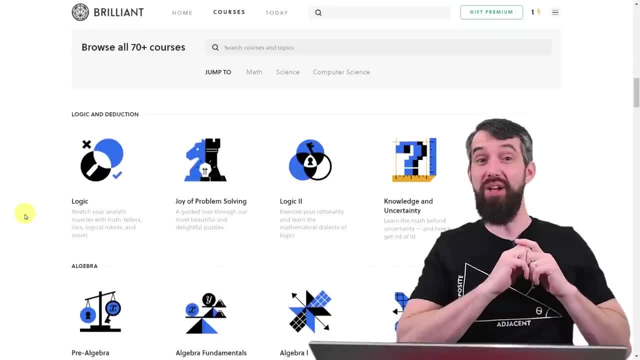 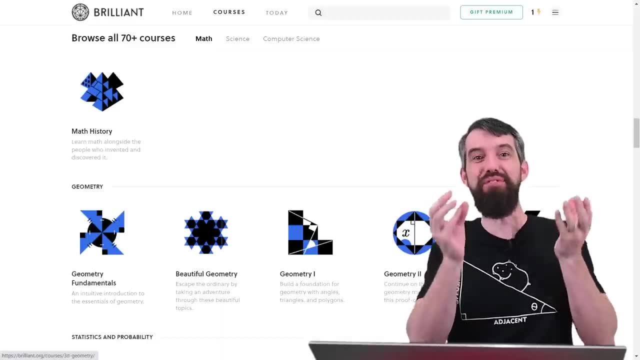 for today's video, which is Brilliant. Brilliant has a whole ton of different courses, but in particular, they have an entire sequence dedicated to geometry and it's just delightfully interactive. For example, if I have two different prisms with the same height and width and length. 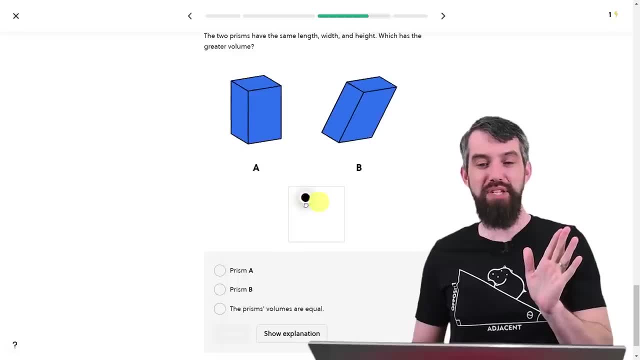 do they have the same volume? Well, as I grab the toggle and sort of move around, I can nicely visualize exactly what the two shapes are And I'm going to naively guess. perhaps I think prism B is going to have a larger amount of volume.